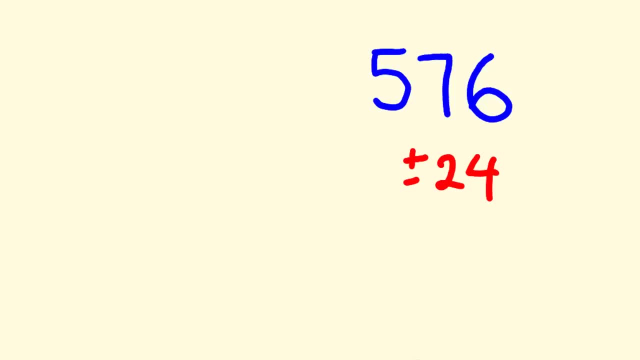 Having said that, I'm probably not going to worry about doing the positive or minus for the rest of these numbers here. I'm just going to put them down as numbers and you can assume that there's a positive or minus there. So I'm going to show you how we do this, and it's going to involve 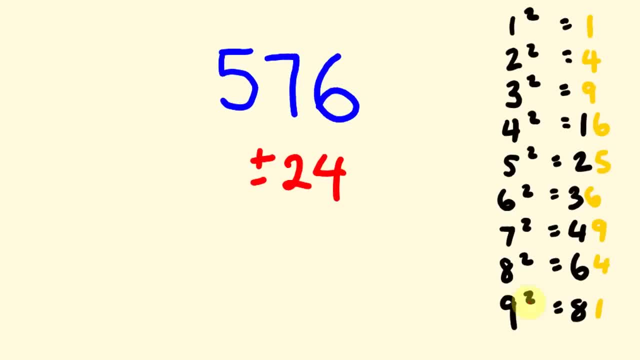 knowing your squares all the way up to. I've done it up to 9, because I think you should probably know 10 squared. I think you should know these already anyway, I think probably most of you would, But you're going to see that I've got jotted down here the squares: 1 squared is 1,, 2 squared is 4,, 3 squared is 9,, 4 squared is 16, and so on and so forth. 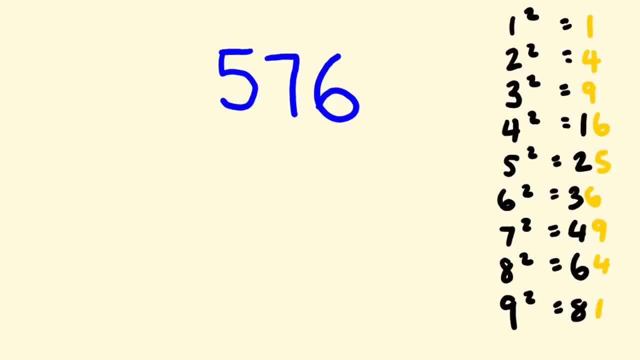 We're going to be using these a fair bit. You're also also going to notice, first off, that I've actually put the units of these in a different color. I'm just going to draw your attention to those actually right now, when we first are working out our answer here. 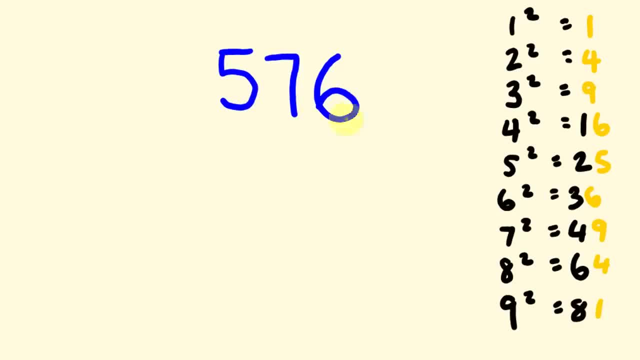 So the way that we do it is as follows. The way we work out the square root of 576 using this is as follows: Okay, So first thing we do is we have a look at this particular unit's answer, the number here. okay, the 6.. 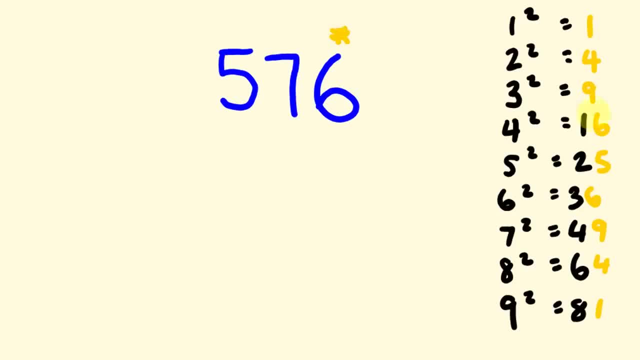 And we're looking for a square root here that corresponds to this, or a square- sorry, a square- that corresponds to this. So 16 does and 36 does And the square root that goes alongside of those we have 4, when we're talking about 16,. 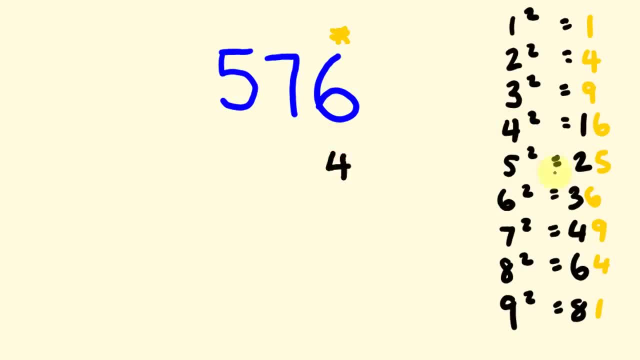 and we have 6 units When we're talking about 36.. So our answer is going to finish in a 4 or a 6. And we're going to work out for sure which one. this is in a little second. But first off, we have to work out now our first digit. 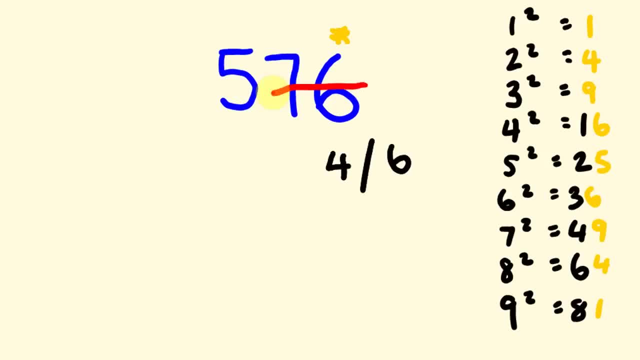 So I'm going to cross out these two digits. it's the next thing we do And we just deal directly now with this 5,. okay, Now we're going to have a look here along here in our square- answers here, and we're looking for a number that occurs. 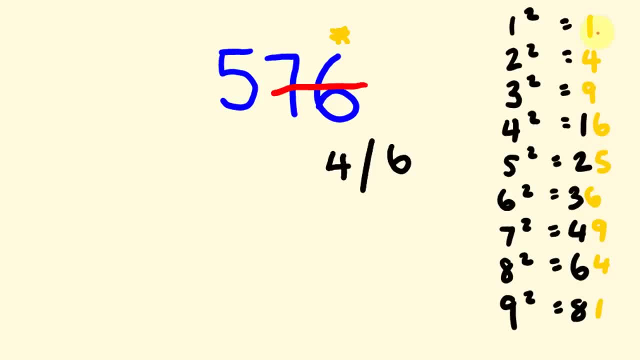 just below 5.. So it's either going to be the number 5 itself or the one closest to 5, which is under okay. So you're going to go along here and you're going to see 1,, 4,, 4's just under 5, and 9's too much. 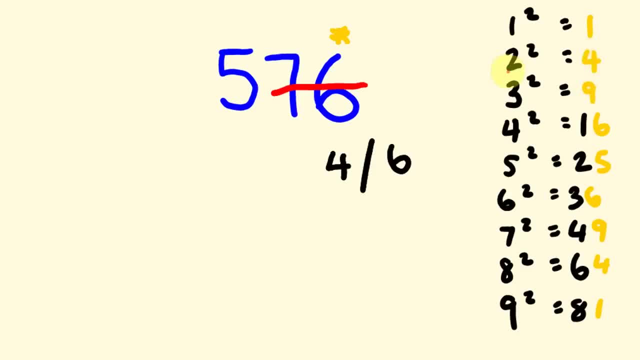 So we're going to be dealing with this? 4.. Now, the square root of 4 is 2. 2's the first part of our answer. okay, Now we're almost there. Now we have to just work out whether or not we're dealing with. is it 24 or 26?? 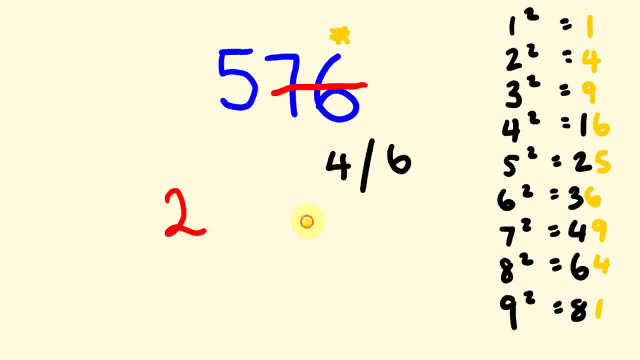 That's our answer, And the way we do this as follows is: we get our 2 here and we just multiply it by the next number up, okay, And I mean the next number up from 2, which is 3.. 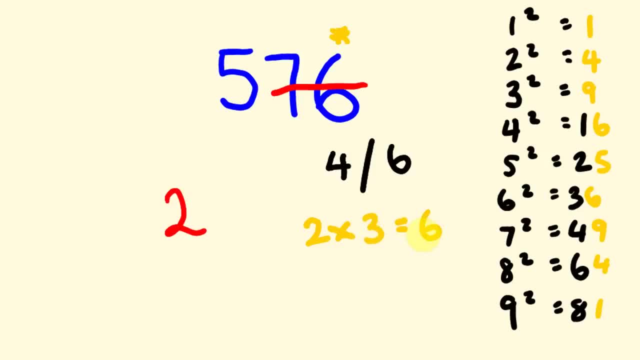 So 2 times 3 equals 6.. Now we have a look at this 6, and pretty much what we do is as follows: If this 5 here is less than this 6,, we choose the lesser number, okay. 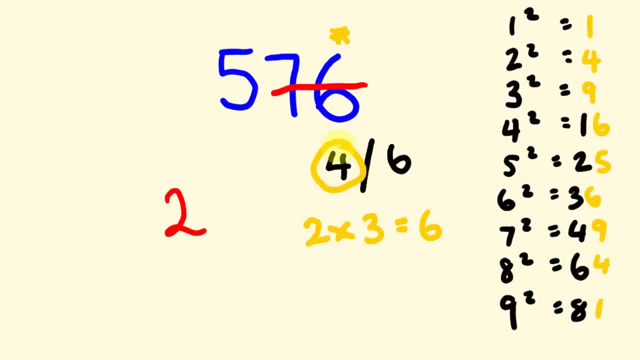 If it was more, we choose the bigger number. okay. So 2 times 3 is 6.. 5 is less than 6, so we choose the lesser number here. So our answer is 24.. Okay, that was a bit of going through. 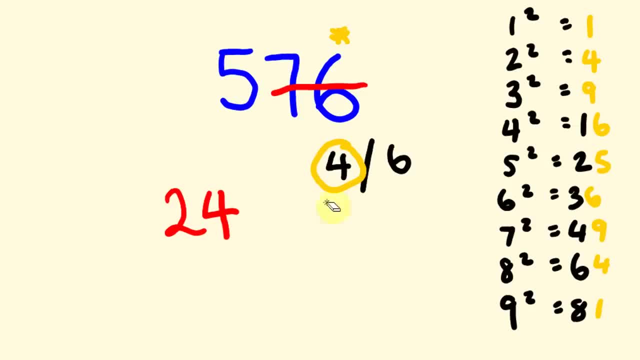 I'll tell you what. we'll go through a couple more of these. You'll pick them up as we go along, And then what I'd recommend is you'll probably be able to start pausing it and giving it a go. 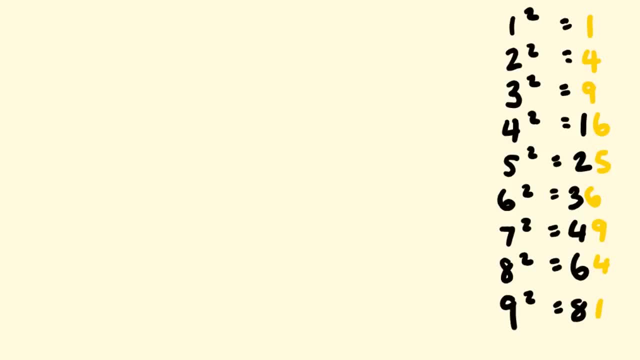 Okay, so let's get into another one of these. So what about? we do 1,849, and we're going to work out the square root of this. So, first off, once again, what we're going to do is we're going to work out the square root of this. 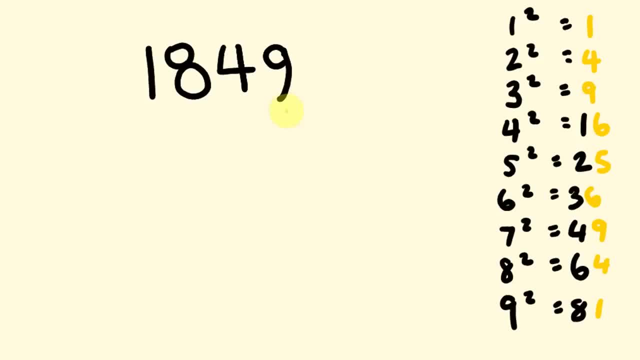 So, first off, once again, what we do is we're looking at this 9 here, Okay, the 9,, and the number that goes along with our 9 could either be a 3 or a 7.. You'll notice, these complementary numbers add up to 10 too, so it's kind of a handy little thing. 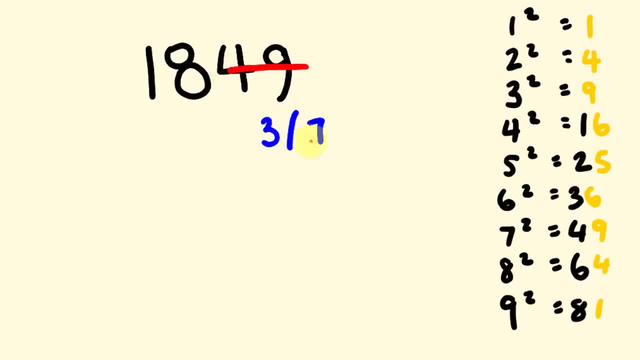 The next thing I do is I cross out these two numbers. Okay, so our answer is going to finish at a 3 or a 7.. Now I look at this: 18.. So 18, and I go down here and I'm looking and 16 just occurs below 18.. 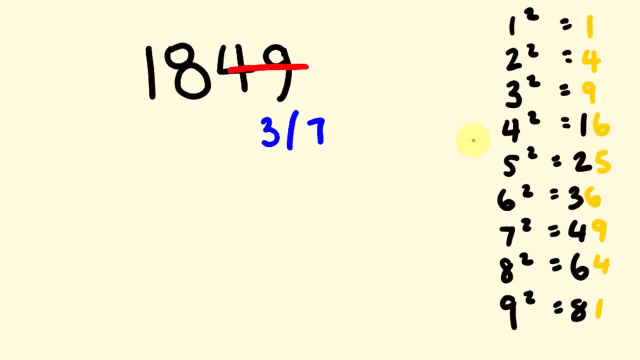 25 is too much. So the square root of 16 is 4.. The first part of our answer is 4.. Okay 4 times 5, okay 4 times 5 is 20.. And now I compare this to 18 here. 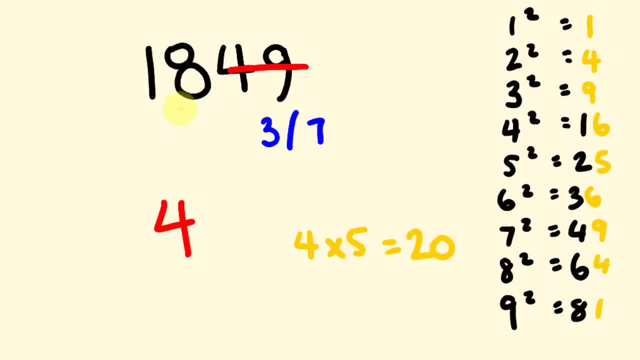 So 18,, as you'll see, is less than 20.. So we choose once again the lesser number. Okay, so our answer is 43.. You get faster and faster and faster at these. Okay, keep practicing them. 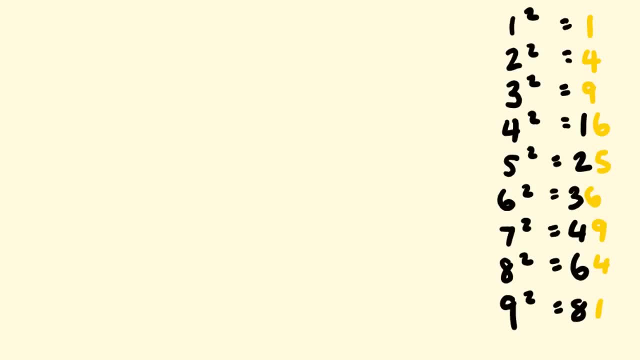 You will get used to doing them, okay. Okay, what about one more of these 3,364.. Okay, pause it, Give it a go. Okay. so looking at the last number here, it could be either a 2 or an 8.. 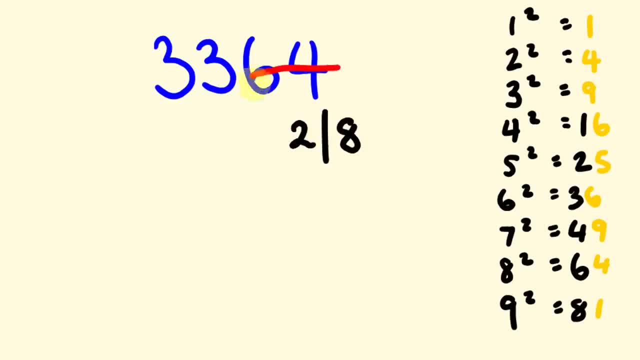 Okay, so let's cross out these two digits here And now. what we do is we are looking for that first digit. Okay, so it's going to be a 5.. Okay, you're probably working that out really, really quickly, okay. 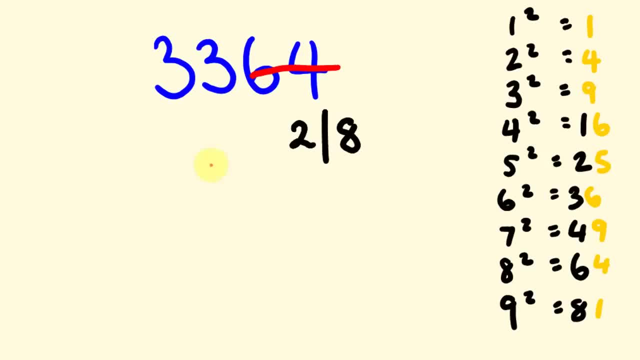 Because 5 times 5 is 25.. 6 times 6 is 36.. That's too much, isn't it? So let's go 5 times 6.. 5 times 6 is 30.. 33 is bigger than 30.. 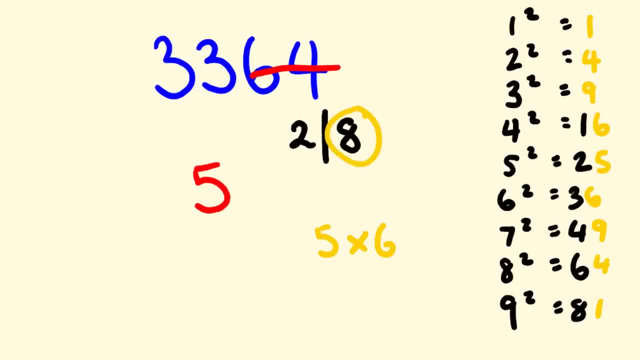 So we're going to choose the bigger number. We have an 8.. So our answer is 58.. Okay, What about another one? What about a bit of a different one? here, We'll do 2025.. Now, this is a nice and easy one, and you'll see why. 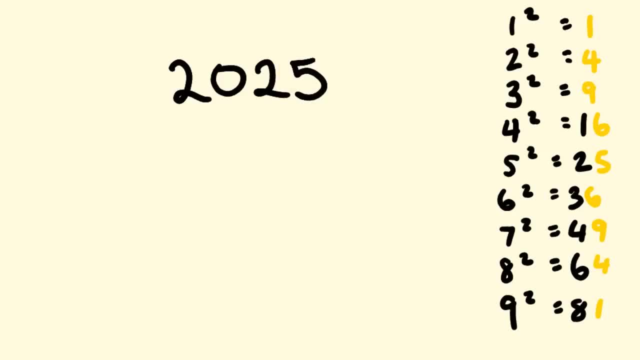 Okay, pause it and give it a go. Okay, so 2025.. You're going to see that it can only be a 5 at the end here, because there's no other option. Okay, cross that out, And then we're looking for the number which is going to be occurring under here. 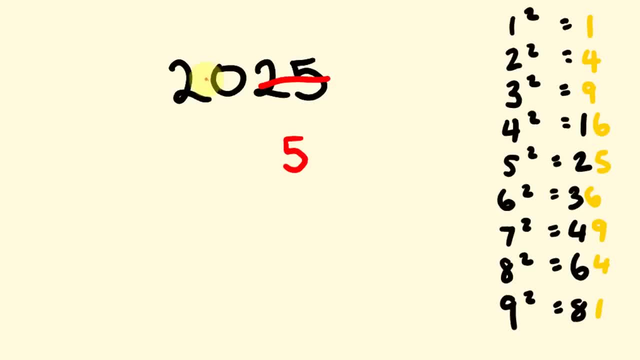 Okay, so 4 squared is going to be 16.. 5 squared is too much, So it's going to be a 4.. But this is our answer, because we don't need to differentiate between whether it's a 5 or. 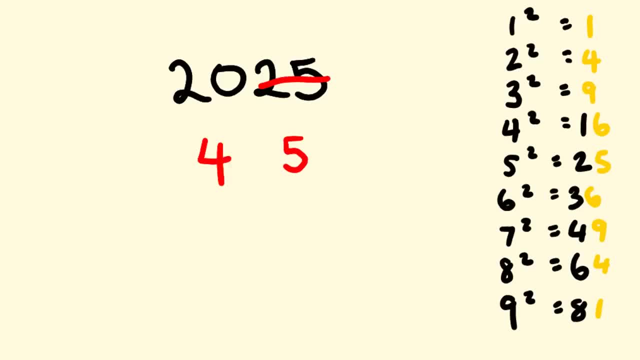 It's just that 5, isn't it? So 45 times 45, that's our answer. Pretty cool, right? Okay, a couple more of these. I've got about three more of these. I'll put them out there. 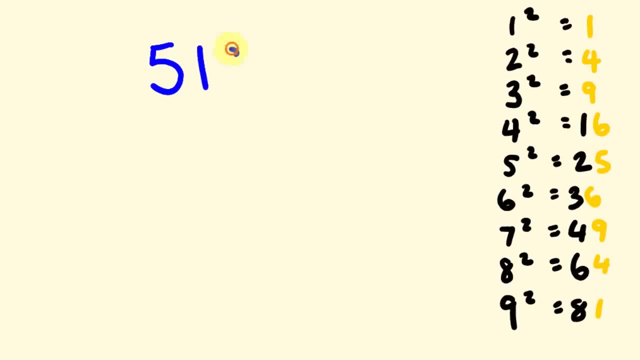 I reckon we can keep practicing them and see how you go. So 5,184.. Okay, So our last number could either be a 2.. Or an 8.. Okay, 7 squared is 49.. So this is going to be a 7.. 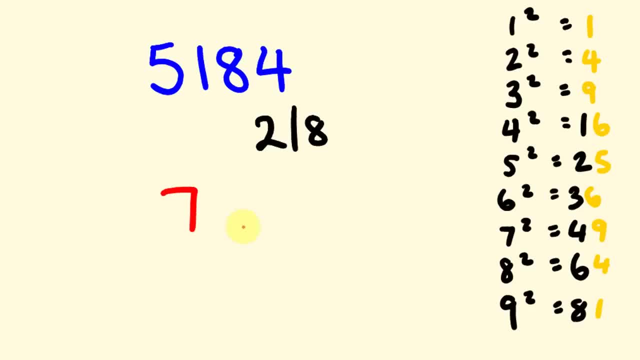 Okay, 7 times 8 is 56. And 56 is 51 is less than 56. So we're going to choose the 2.. Okay, This is how I start doing these in my head. I'm going to start doing them more and more like this. 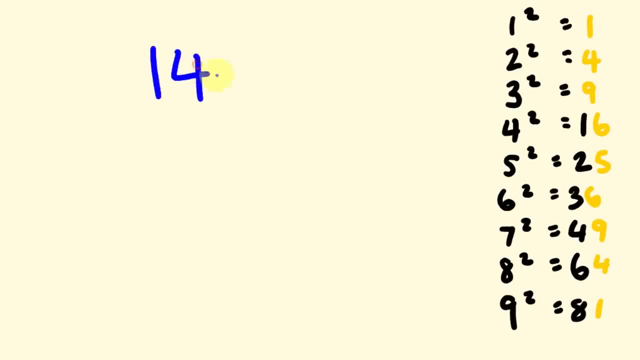 I'm going to do the rest of them like that, I reckon. So what about 1,444?? Okay, So the last number here could be a 2. Or it could be an 8.. Okay, So 14.. 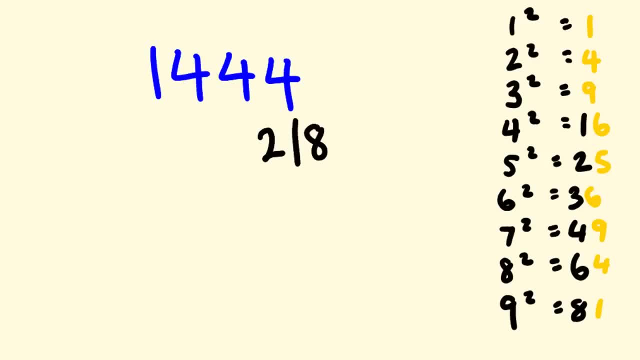 16 squared is 4. squared is too much, 3 squared is good, So it's going to be a 3.. 3 fours are 12.. 14 is greater than 12. So we're going to choose the greater number, which is an 8.. 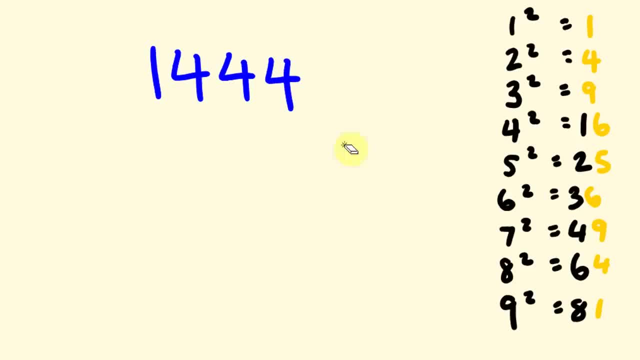 38.. All right, Lucky last one out of all of them is 8,281.. Okay, So, as you see here, 81.. Well, 81.. I'm only going to look at the last number here. I know it's sort of tempting to go 81,. hey, wait a second, that's 9.. 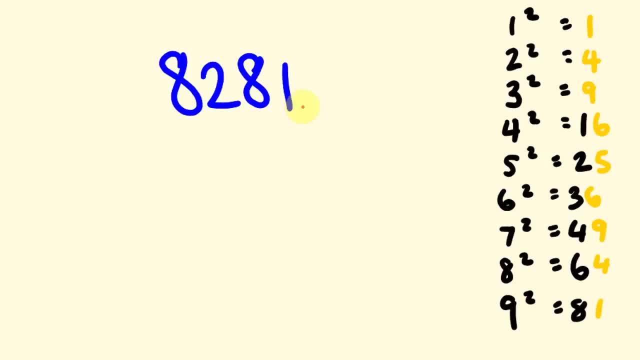 I'm only going to look at the last digit here, So 81.. It could be a 1 or a 9. Okay, So what we'll do now is We'll cross that out And 82. Okay. 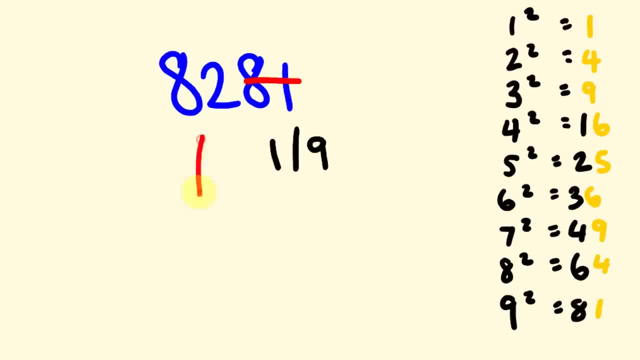 So 82.. Once again, this is going to be a 9.. Okay, Well, it's not going to be a 9, because it's not necessarily a 9.. So we've got 9.. Okay, So 9 times 10 is 90.. 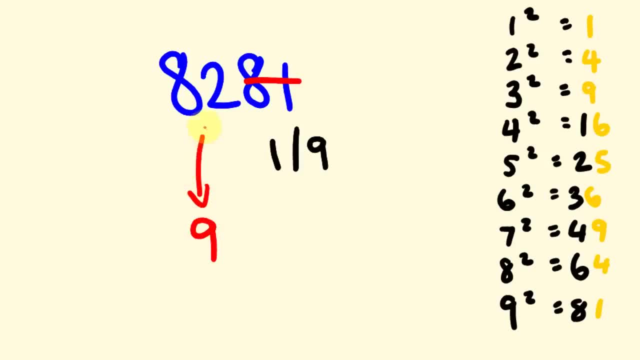 82 is less than 90. So we're going to choose a lesser value. We've got 91. Anyway, what did you think of that particular trick there? It's not a bad trick. Okay, It does take a bit of getting used to, but once you get used to it it's actually fairly. 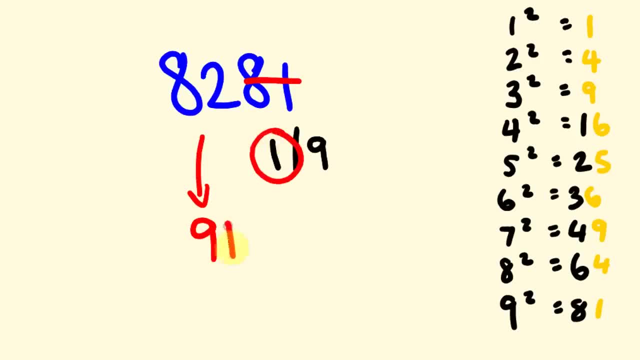